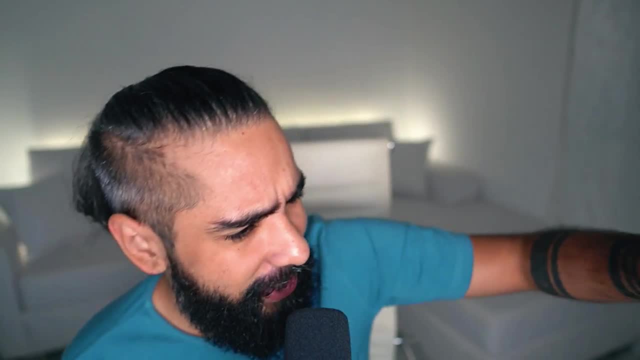 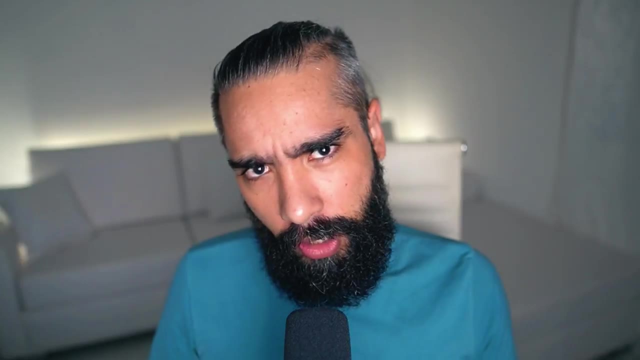 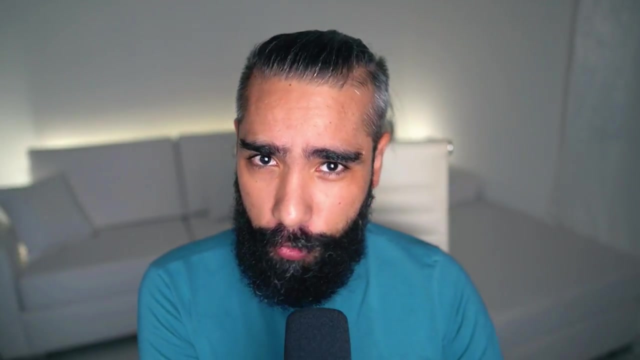 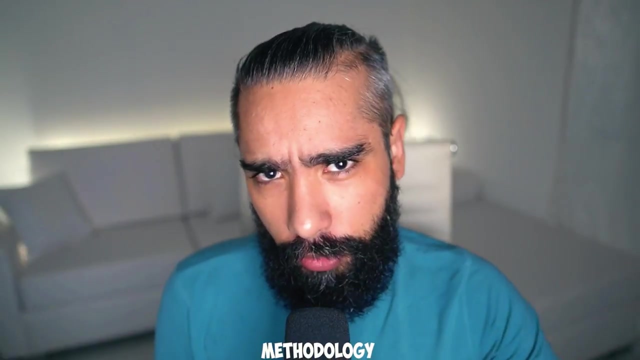 Innovate or die. Tech companies, or even companies in other industries, want to remain relevant in an ever-changing environment, ever-changing industry. These companies- small, big, medium companies- want to push out products, their products forward as fast as possible in a short time frame, And the agile software development methodology was developed exactly for this reason. 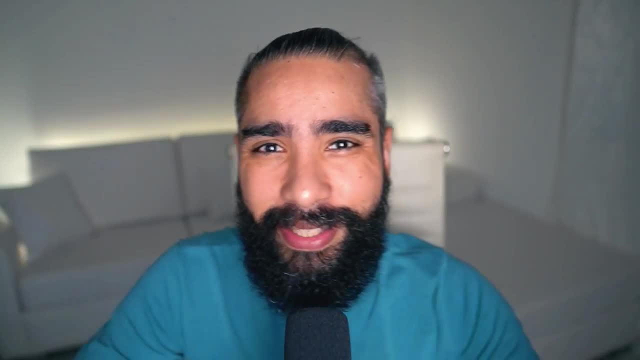 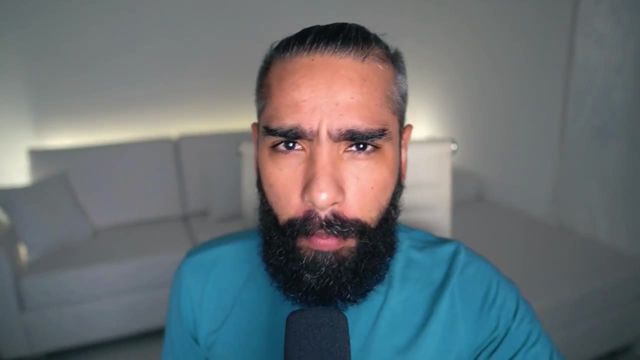 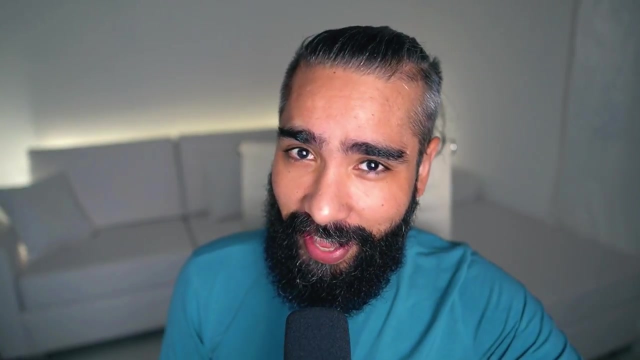 Rapid development, rapid deployment, while still maximizing value. Some of you wanted me to talk about the six phases of the agile software development life cycle with real-life examples, And this is exactly what we'll cover today. Let's get to the chase. 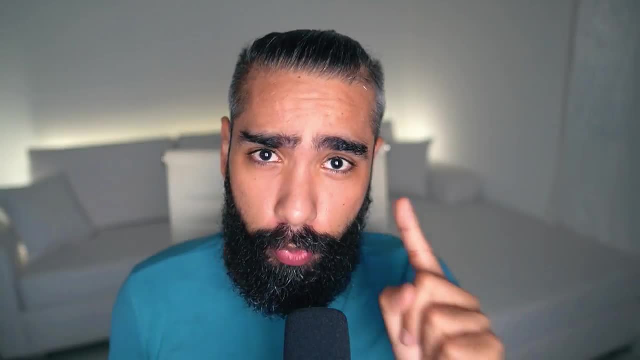 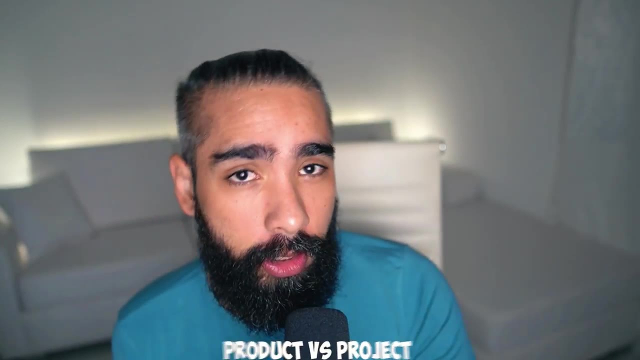 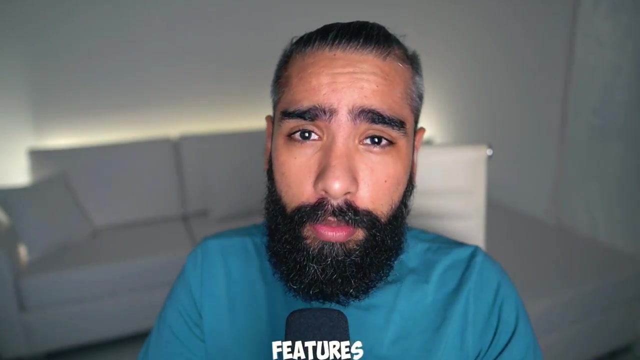 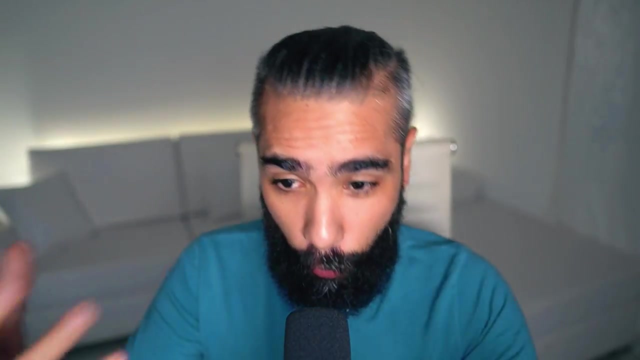 Phase one, concept or objective. Here the product owner will define the scope of a project. Now, there's two types of scopes: There's the product scope and the project Scope. It's really important to know the difference. Product scope is defined as the functions, features that characterize a product or service, Whereas the project scope is the work that needs to be done in order to deliver that service. according to the product scope, the functions, the features. 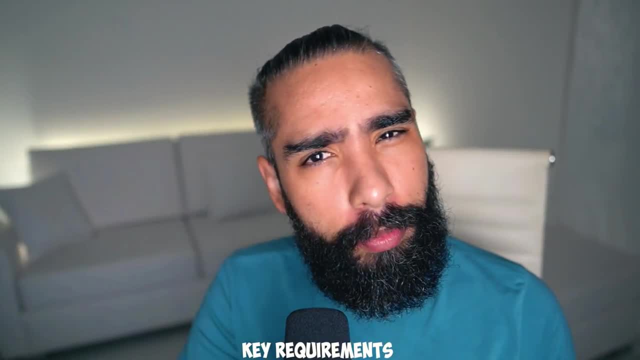 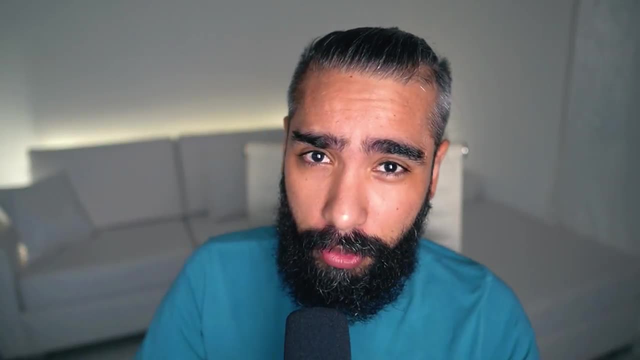 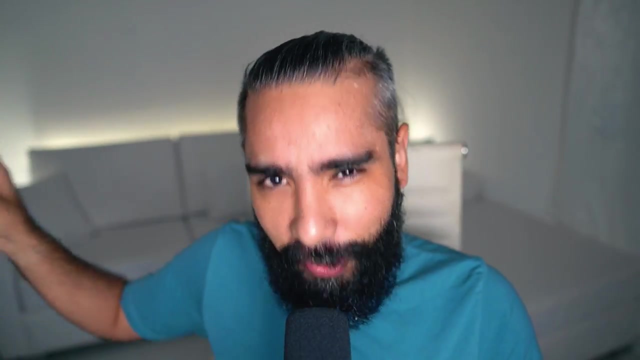 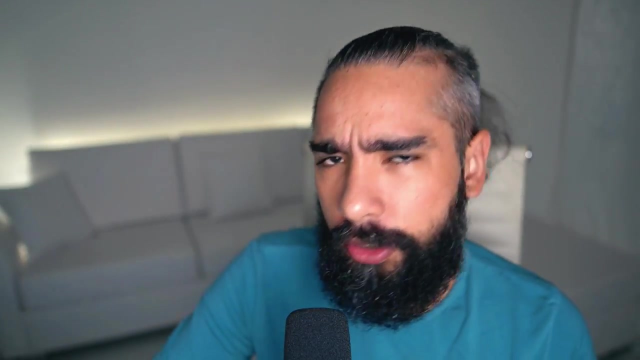 Here the product owner and the client will talk about the key requirements that need to be included in the product or service, And these requirements, functions, features, will be included in the documentation. Now, at this stage, if you are using the waterfall model- the old, the classic waterfall model- you would write an extensive documentation really detailing all the features, all the functions. 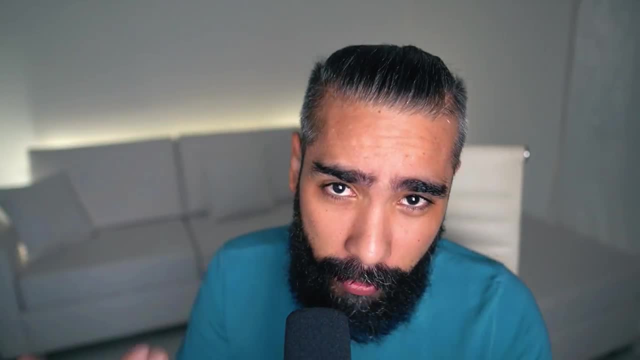 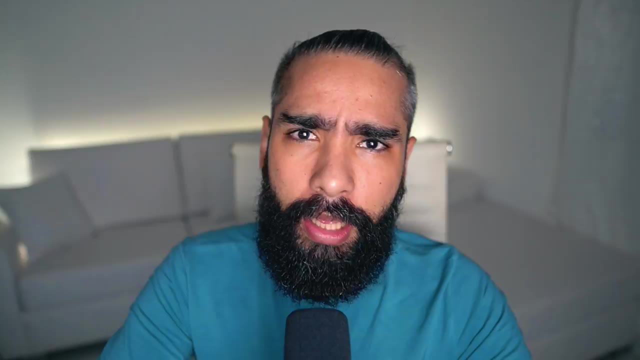 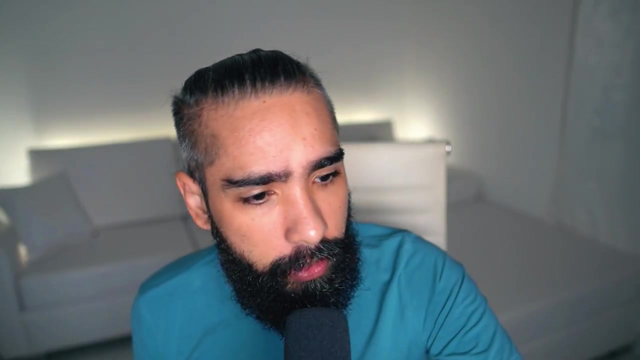 But in agile it's not recommended to do that. It's recommended to write the minimum in terms of documentation, requirements, function, how the product will and service will look like, the end result of a product or service, Minimum requirements And documentation, because we can always add it at the latest stage. 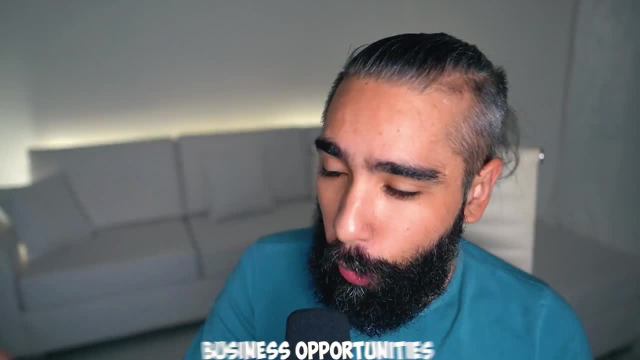 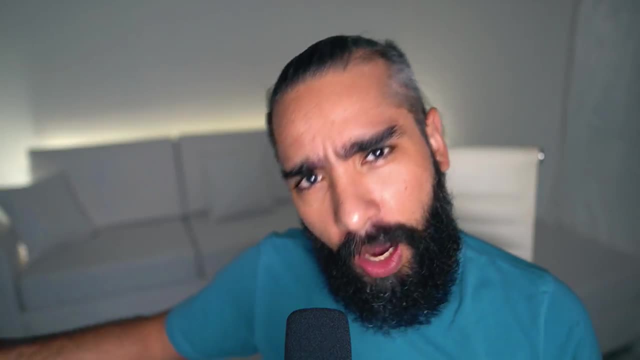 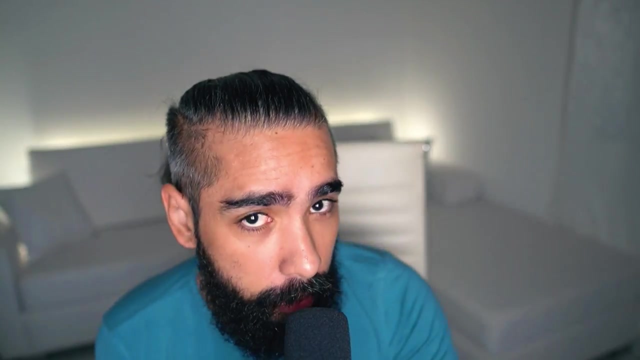 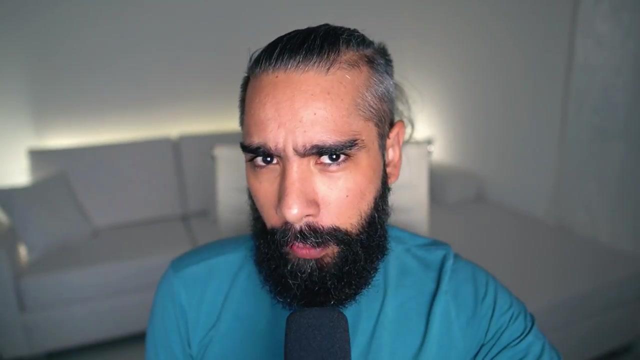 The product owner will also define the business opportunities and the time required to complete this project, Now extremely important. Some product owners miss this part completely. I feel that is the most important part of a project. a product owner needs to define and really understand the problem or problems we are trying to resolve, to solve for the customer, for the end user. When we know the challenges, We are trying to resolve to solve for the customer, for the end user. When we know the challenges, We are trying to resolve to solve for the end user, for the end user. When we know the challenges. 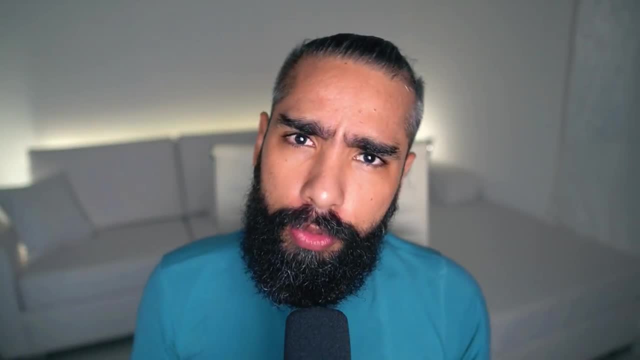 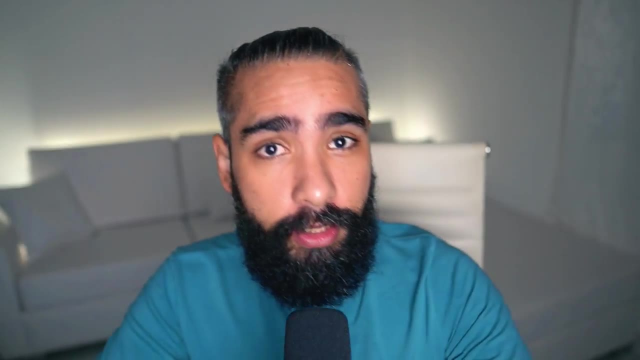 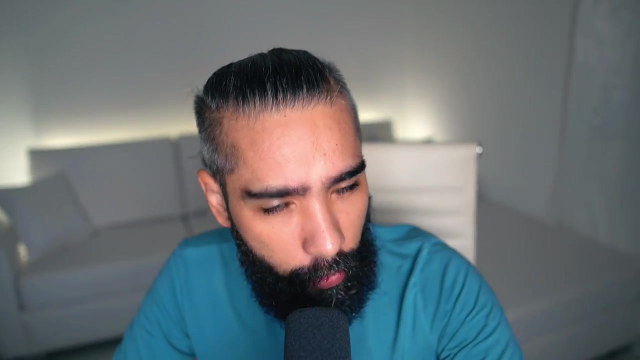 The challenges of the end user, the needs, the wants of the user, will be able to correctly or better prioritize functions and features to solve these problems. give solutions to the end user Because, at the end of the day we are working, we are building something that the user will want to use. 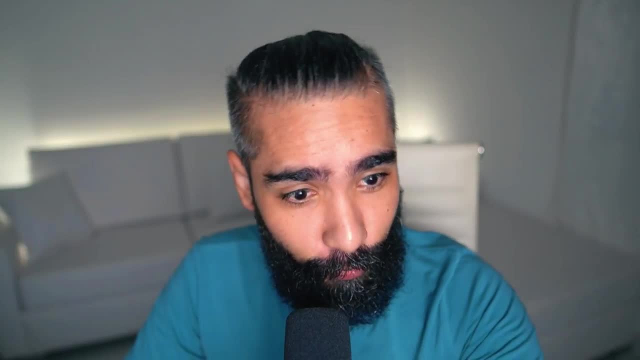 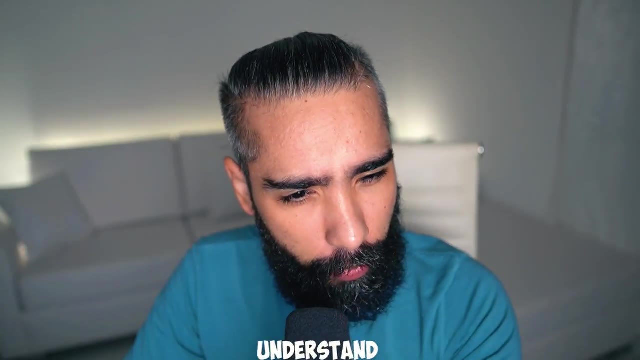 That's the main goal And to know that. we need to know what the user wants And to know what your user wants. we need to be able to really understand the user, what kind of problems the user is currently facing right now, And we come in and fix these problems. 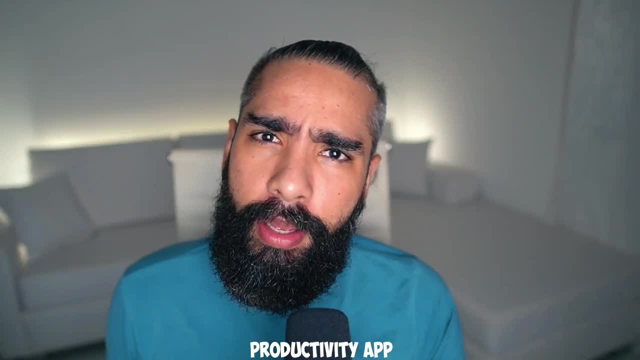 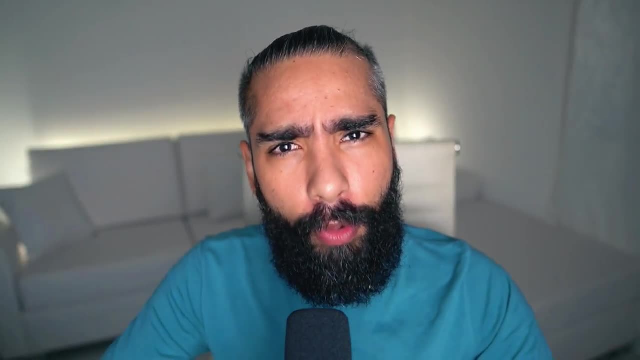 As an example here maybe we are trying to build a productivity app, an app which will allow you to track all the things that you need to do during the day or even after. Maybe three columns comes from default. The application opens with three columns today, tomorrow. 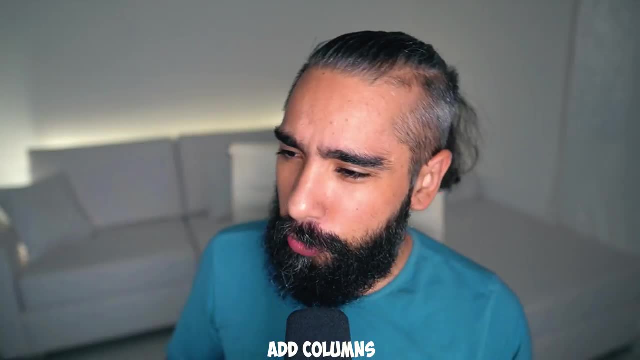 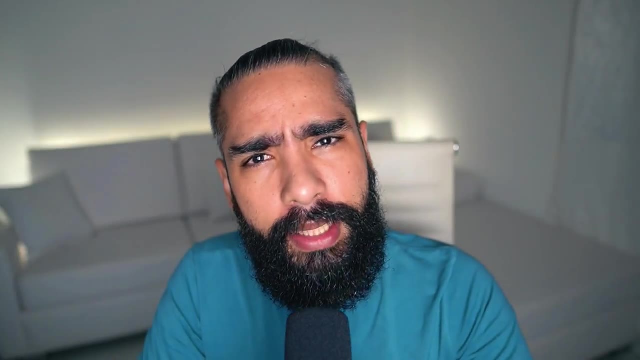 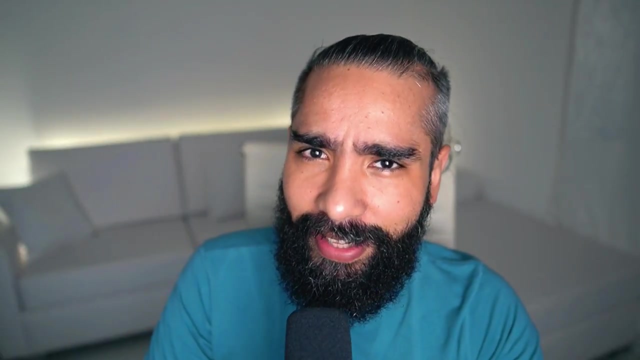 Later maybe the option to add some more columns, the option to create items, move the items from one column to the other, Basic features, And that we are only talking about basic features At this stage. we can add other features and functionality later. We can talk about that later. 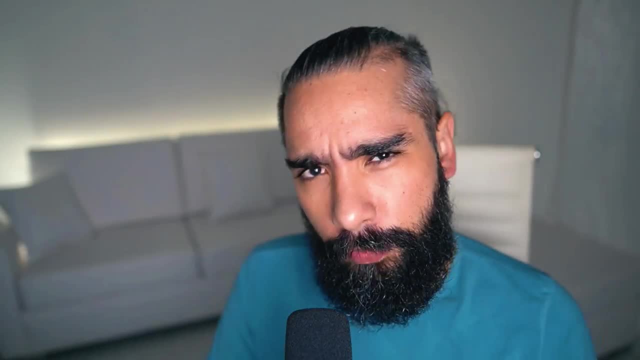 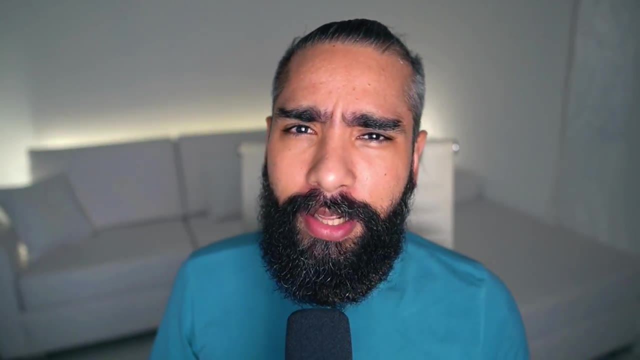 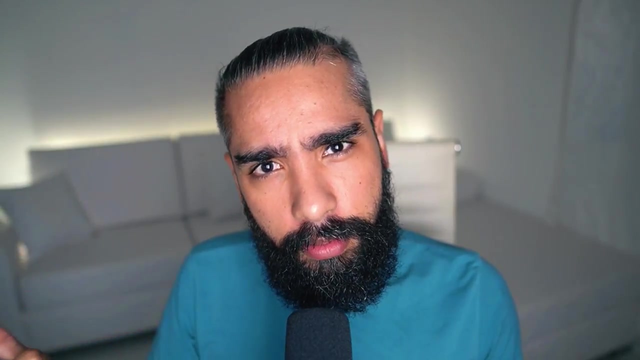 The next phase is the inception phase. The goal, the purpose of this phase is to just do enough work to get your team going into the right direction. Here the team should be ready to experiment, To start, to start to start building prototypes on the requirements that we agreed on in the previous phase. 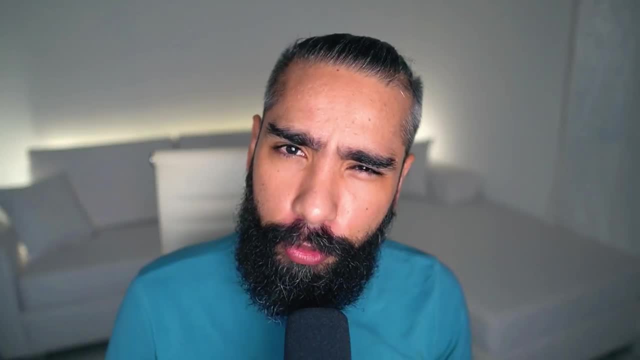 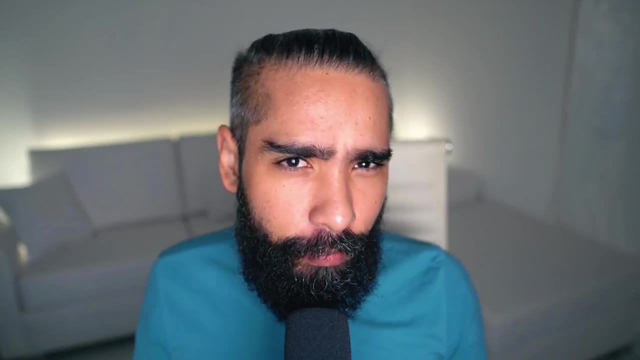 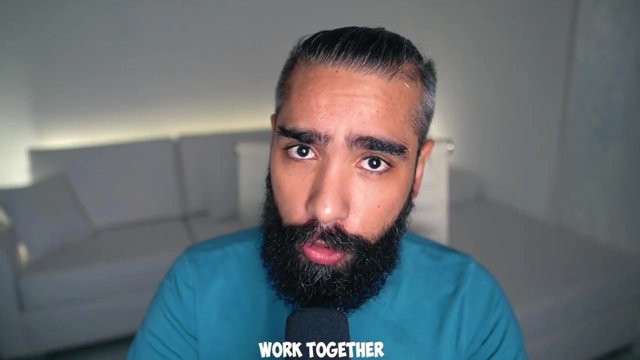 The number one thing the product owner needs to do in this phase is actually build a team, And it's highly recommended that the product owner tries to get the best possible candidates for the team. Developers, testers, designers and everyone, including the product owner, need to work together. 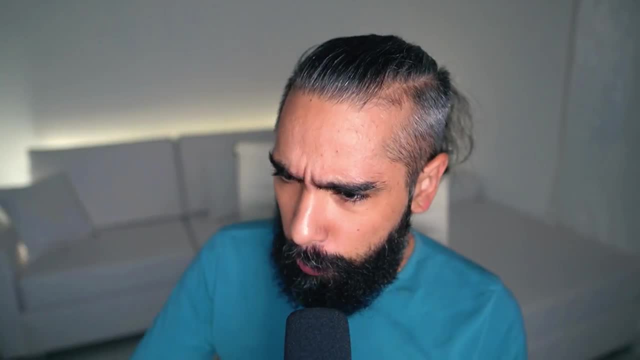 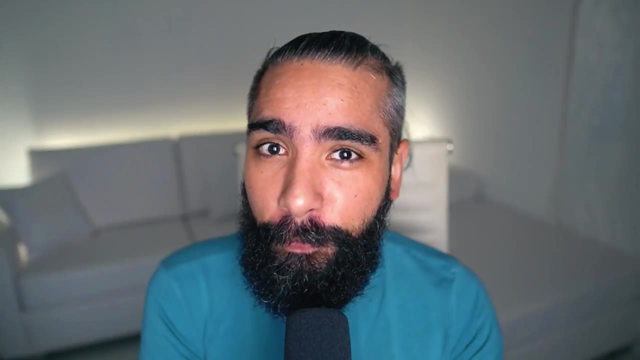 They need to work together to build a mock-up, a prototype, build the project architecture and give them the right tools And then give this mock-up to the client, to the stakeholders, and gather feedback. The more feedback we get, the better. 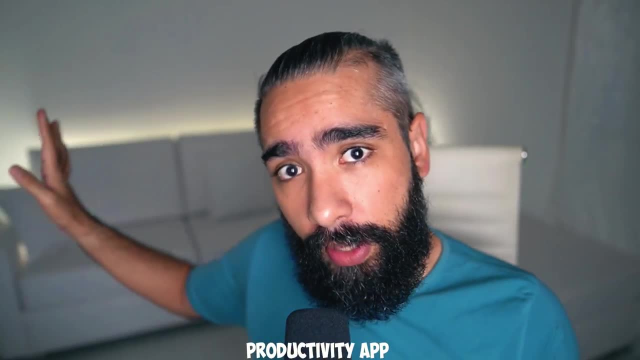 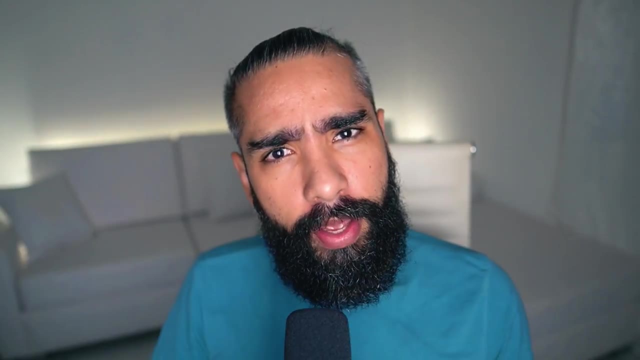 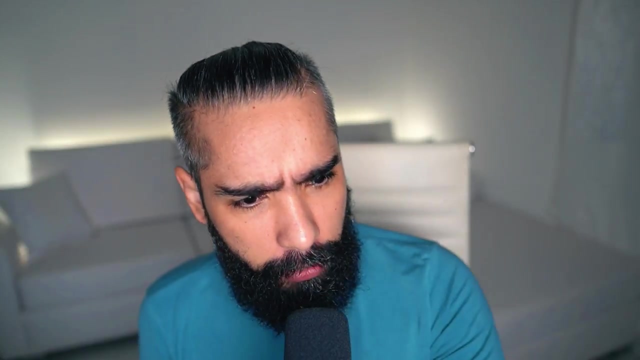 And using the example we talked about previously, the productivity app, the team will build a prototype that can be given to clients, stakeholders, so that they can start adding stuff to the app, adding columns, adding items, start tracking their to-do lists for the day and really give feedback on what they like about the application- maybe the design, the functionalities, what they would like to have. 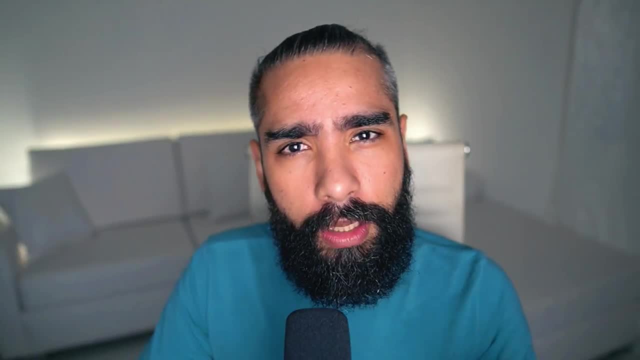 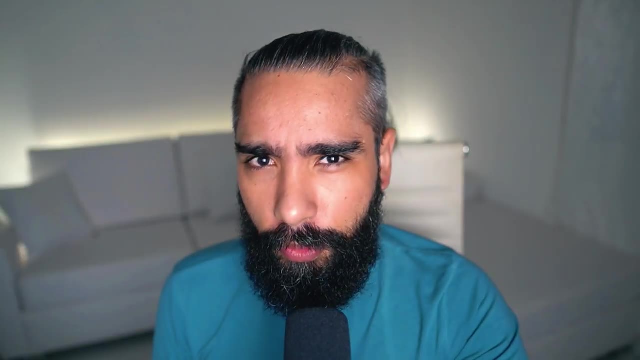 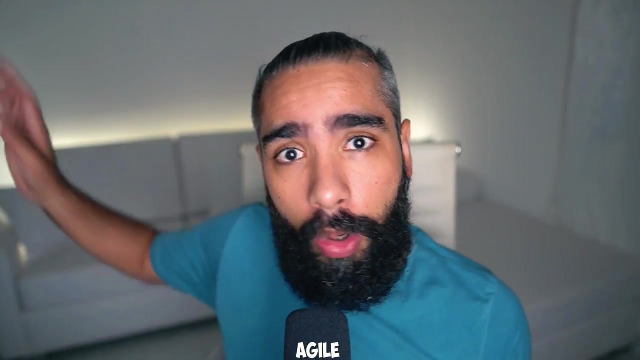 like to improve. we really want feedback from stakeholders, the client, because our goal here is to build the best possible application in terms of value that will be given to the user, to the customer, and to do that we need feedback. that's the whole purpose of doing agile, not the 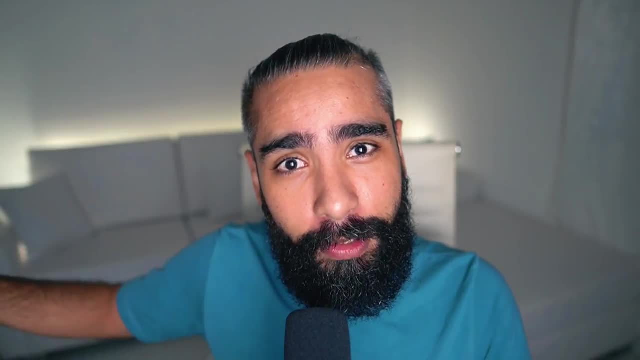 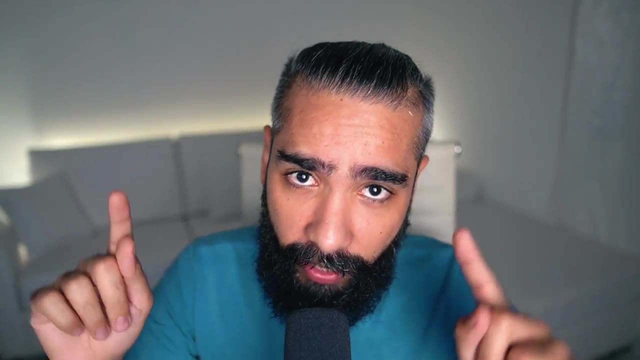 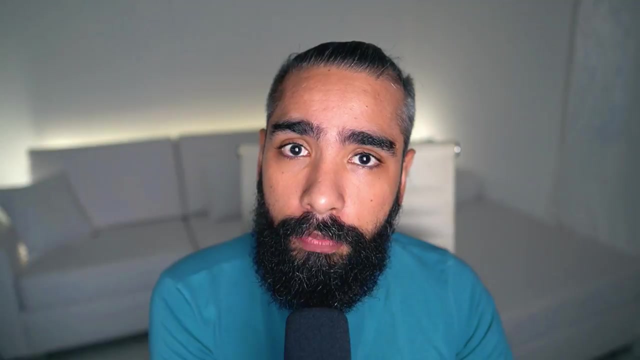 waterfall model where we build something for one year based on requirements that was defined one year ago, without no feedback whatsoever, no client involvement, nope. in agile, constant feedback, incremental approach, we get feedback, we develop, we fix something, we improve something, we get feedback, we improve some other thing, and it goes on and on until the product is perfect, but it will never be perfect. the next phase is the iteration phase, or the construction phase, where we actually build the application which will be released to customers later on. now, in this phase, the, the, the team, the whole team, including the product owner, will sit together to convert these requirements. 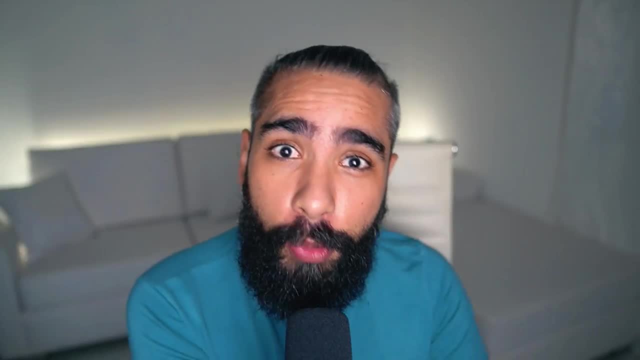 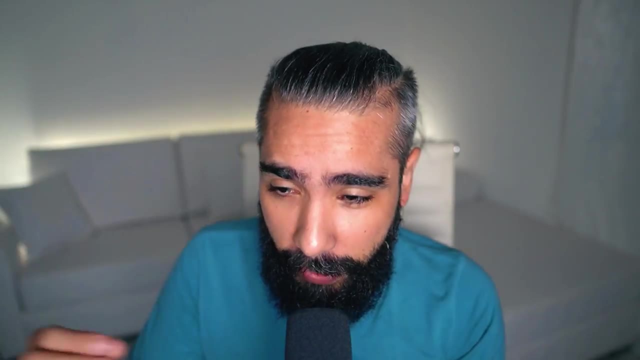 the mock-up that we did, the product that we did into actual code, into a working application, and it shouldn't be a full, flat application with all the features and functionalities. nope, minimum that we can put to the market that will satisfy the customer should be done. our goal here is to release. 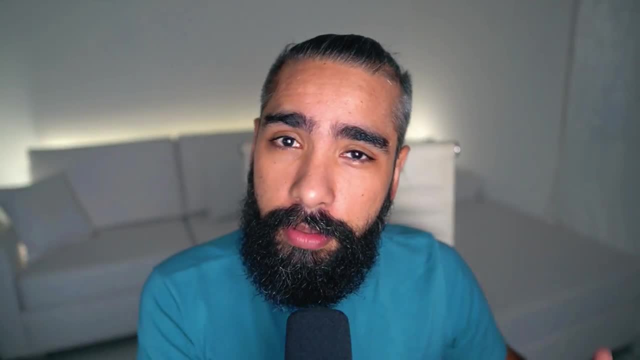 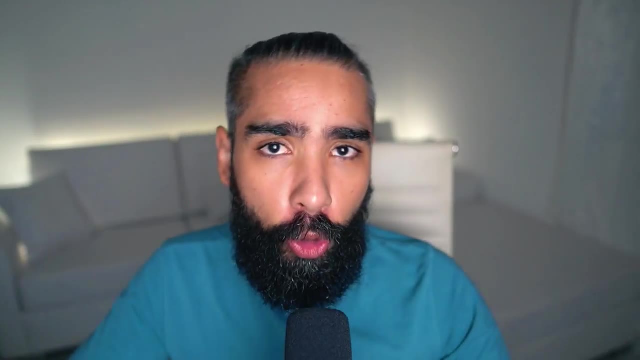 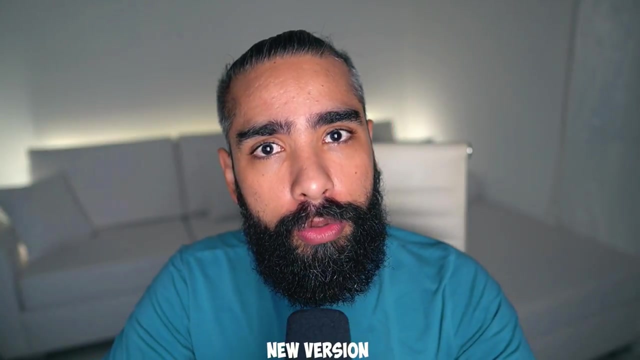 something as fast as possible while still maximizing value. our goal is to constantly be releasing stuff, learning, gathering feedback, learning from this feedback, improving the item, the product application, and then releasing a new version, gathering feedback, learning, releasing a new version, and it goes on and on. you should always in this phase. 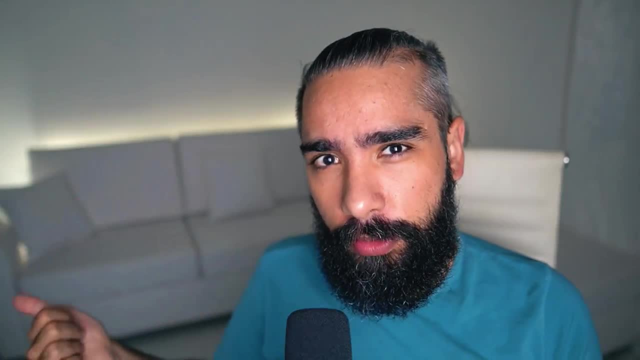 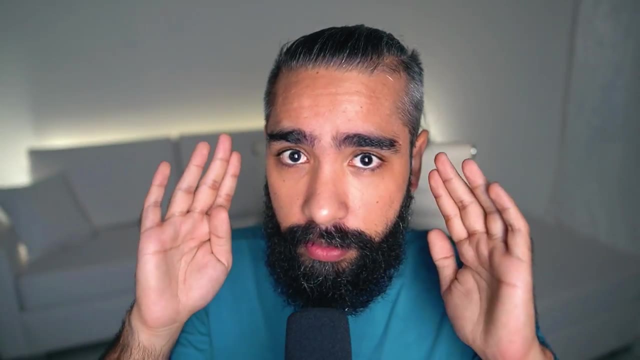 keep in mind the problem that we defined in the concept phase. remember we defined the problem and we were trying to solve this problem, give a solution to this problem with an application. so always have this in mind when building the actual application. now, In this phase, we already have a prototype. so requirements: we need to actually write code. 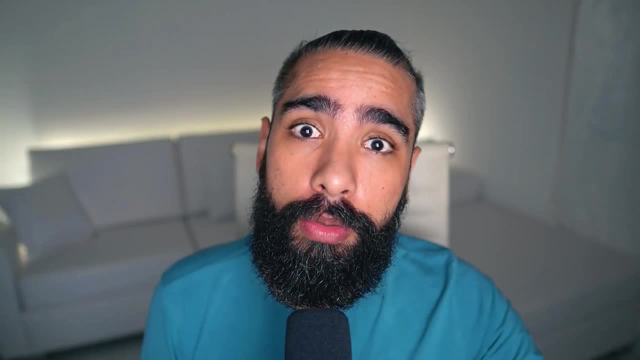 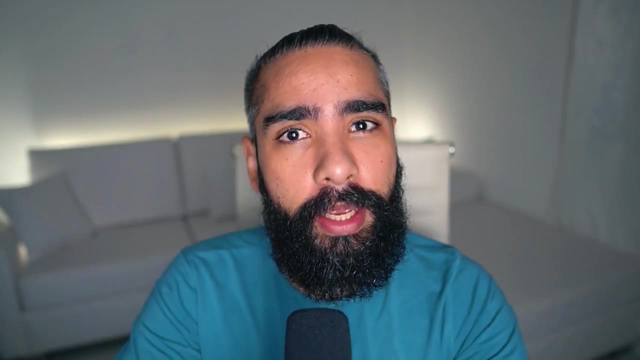 and build a working application that we can give to customers, but maybe not all customers. Maybe we can get some VIP, some special, some beta customers that can use the application. that everyone, some beta users, some VIP customers that can use the application. 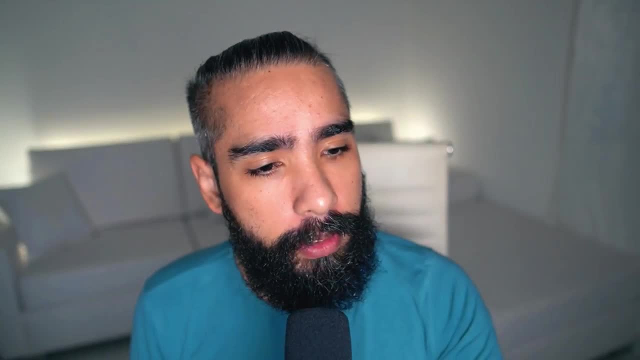 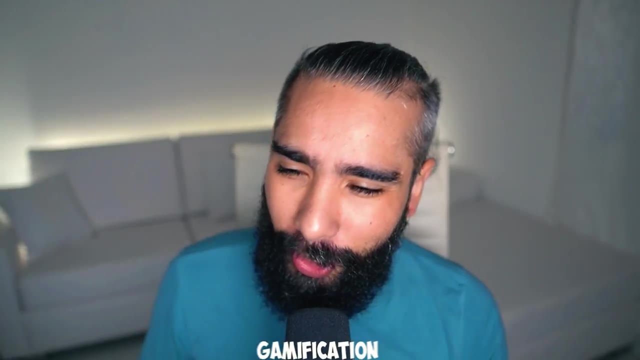 Let's say, in our example, the productivity app. they can use the application. they will give feedback like: okay, the design needs to be changed. Maybe we can add some gamification and make it more exciting to complete tasks in the application. 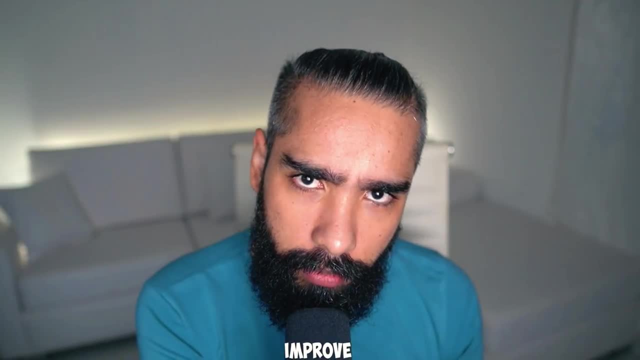 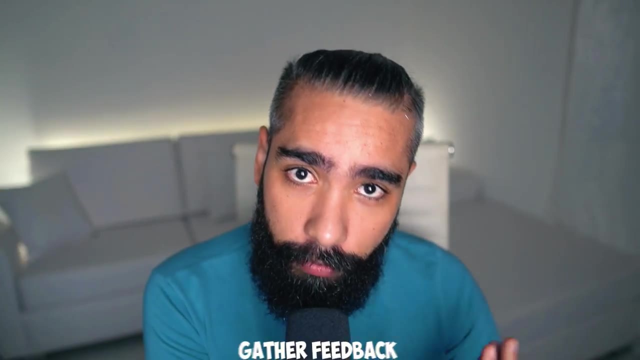 All this feedback. we get this feedback, we improve the application, We have a problem and solution in mind that we defined previously and we release it to the users and we gather feedback again and we improve it. and it goes on and on. That's the whole iteration phase. 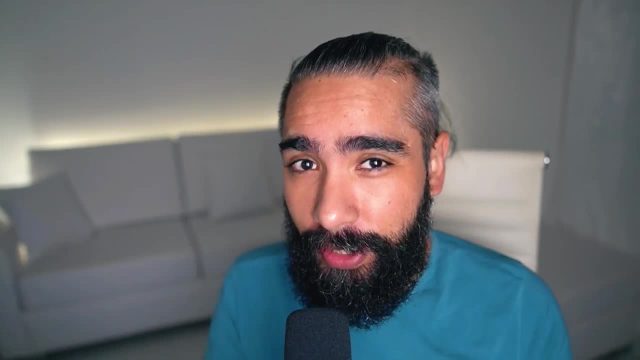 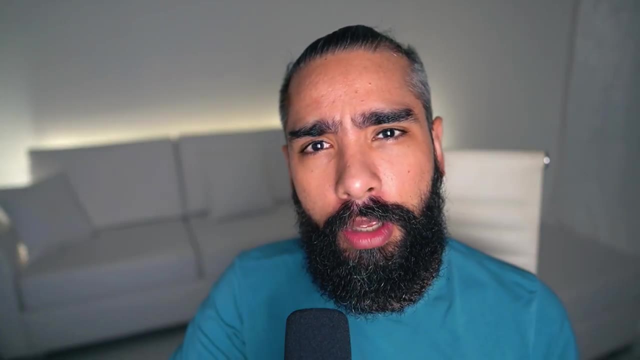 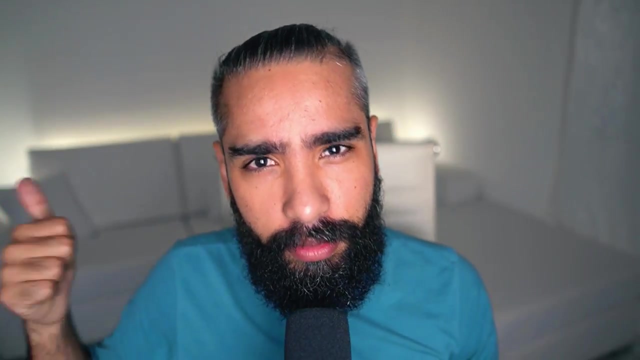 The next phase is the release phase. We are now ready to release the application. Maybe the next iteration iteration we talk- The previous- will be the release iteration. The code has been done. It has been tested. We have ensured that the requirements- all the acceptance criteria defined previously- are being met. 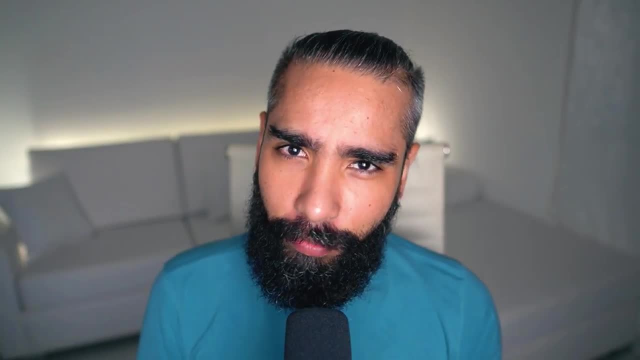 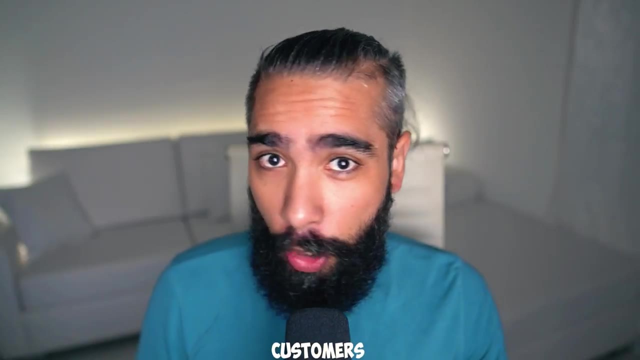 We got the feedback from the beta users. We really like the feedback that we got. They really like the application and we are ready to release it to the actual customers. We ensure here that the environment, the production environment, has been set up. 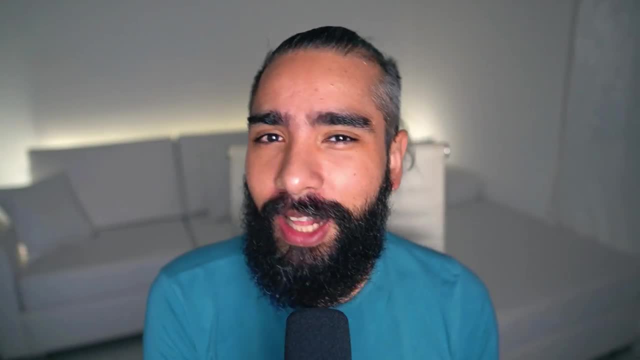 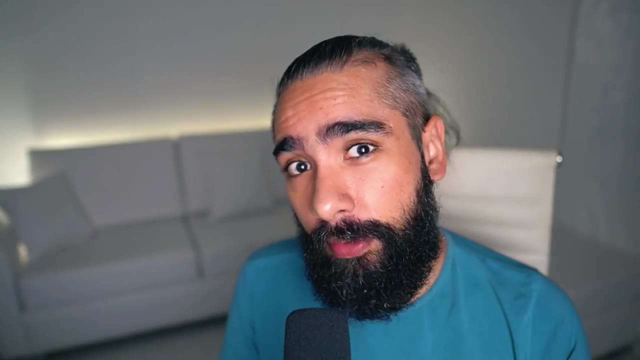 It's stable. We have tested all the code. The functionalities are working, Everything is good and we are ready to release. So this step includes testing debugging, which may result in having bugs, defects, which need to be fixed by the development team prior to the release. 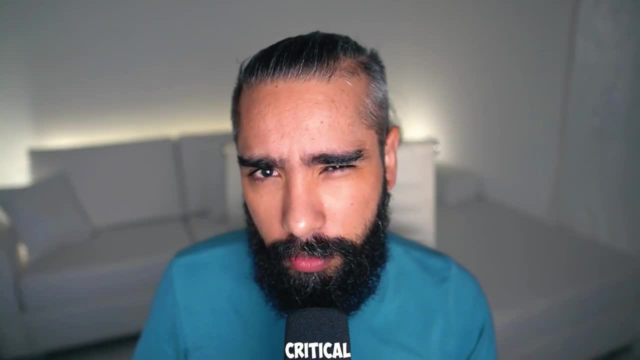 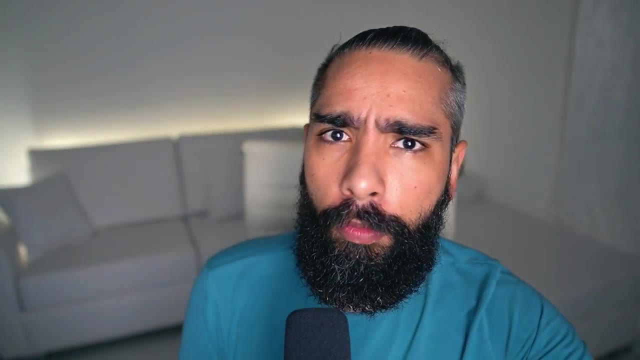 And once we've fixed all the bugs, or at least the critical ones, and we are ready to deploy it to production, we need, prior to that, prior to starting it, application for the customers. we need to ensure that the application has some sort of documentation. 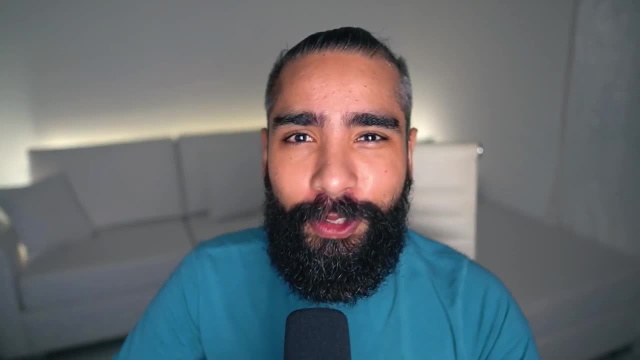 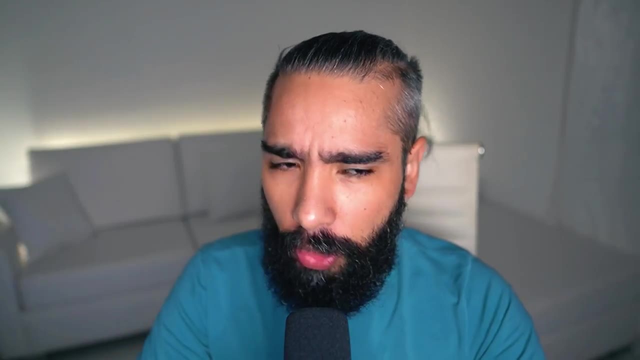 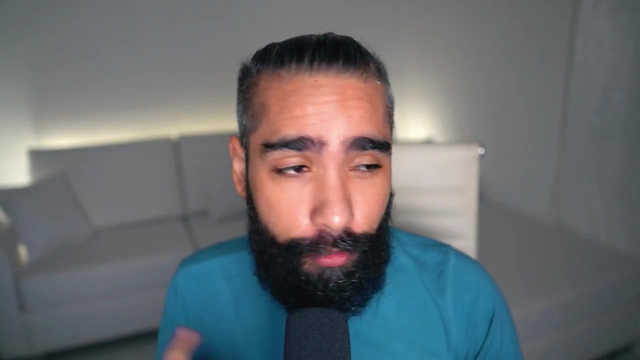 the customer needs to be able to navigate through a tutorial or something to know how to use the application. And once all these things are in check, everything is done, we deploy it to production and congratulations: your application is now released. It's not the final version.